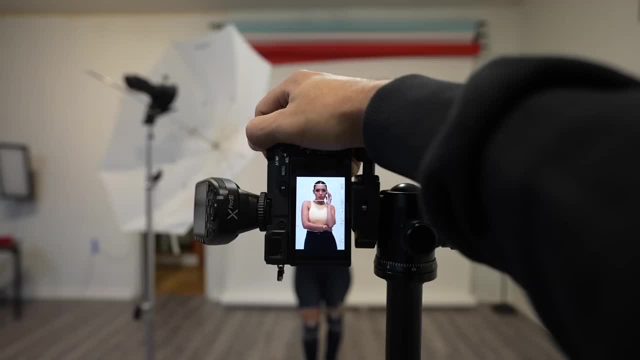 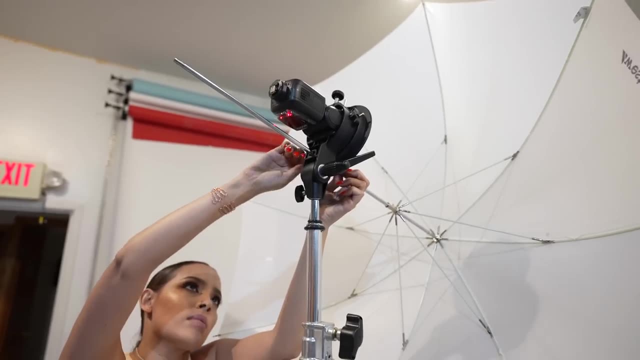 and bring the best out of your camera. Let me show you how it's done. I'm going to show you how to take some professional portraits using my cheap camera: only one flash and a cheap $20 umbrella. I'm going to go over the gear specifics and the settings that I used later. 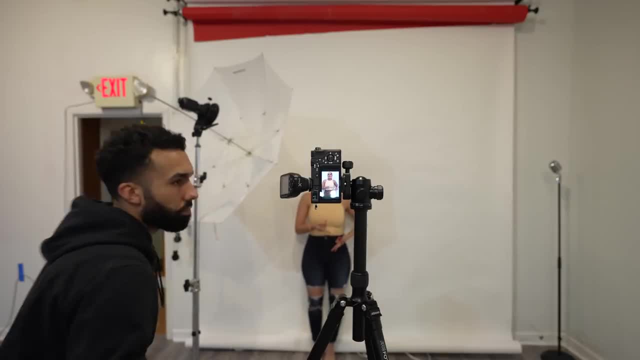 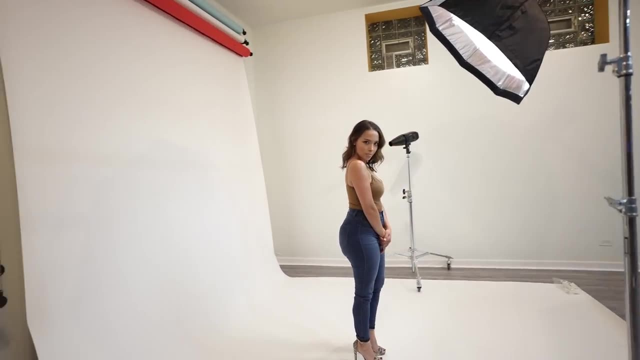 on in the video. So let's start with the most important part: light position. I made a whole video on this topic and I highly recommend you check it out. I'll leave a link down below. But personally I think light looks best when it comes from a 45 degree angle, slightly angled down. 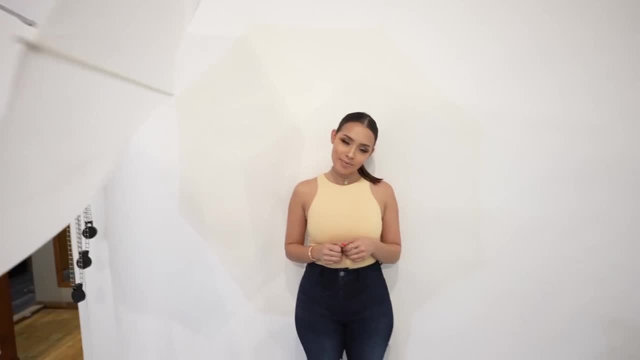 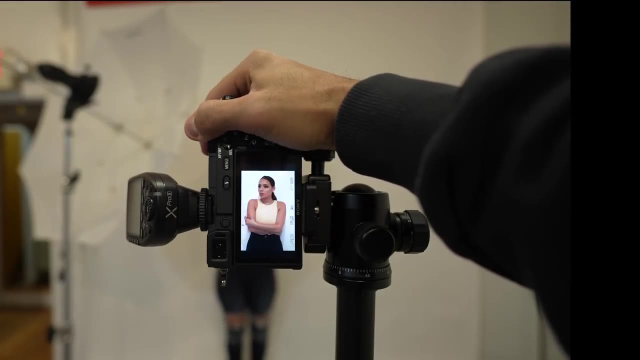 towards the model Things that you need to have on point. You want to have it as close as possible so that you can get the softest light quality, And you want to make sure that you have a catch light in the eye. That's the key. You want to make sure that you have a catch light in the eye. That's. 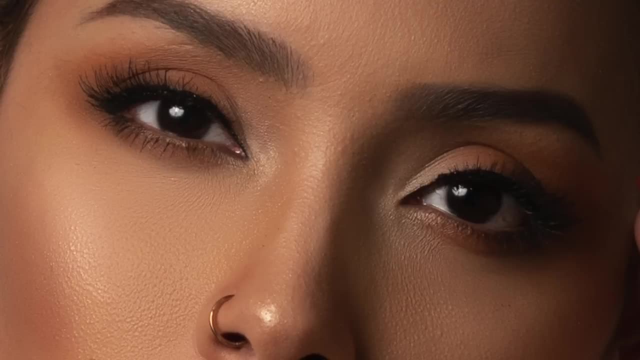 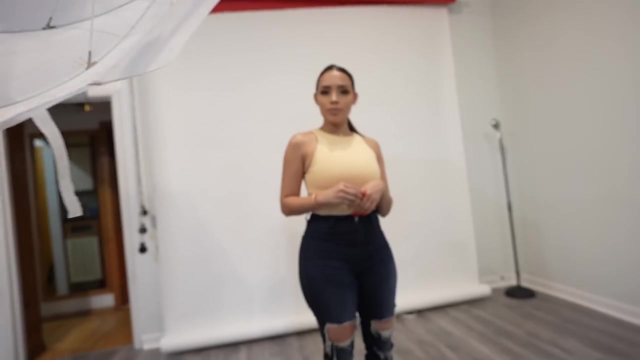 a reflection of the umbrella in the eye. If you don't get that, you have to make adjustments. until you do, I'm going to show you that changing the model's distance from the background will make a huge difference in the outcome. First, let's put her up against the white backdrop. When you 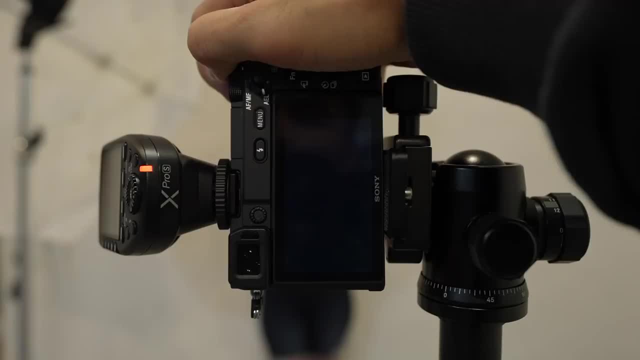 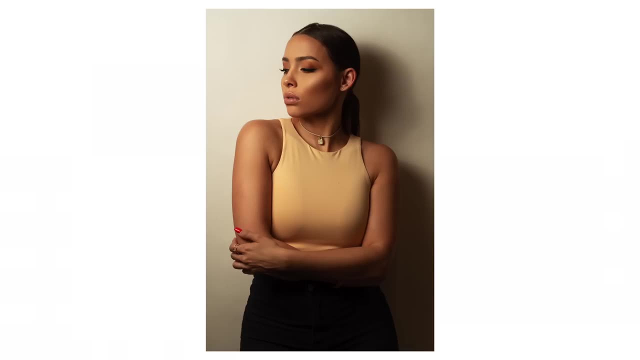 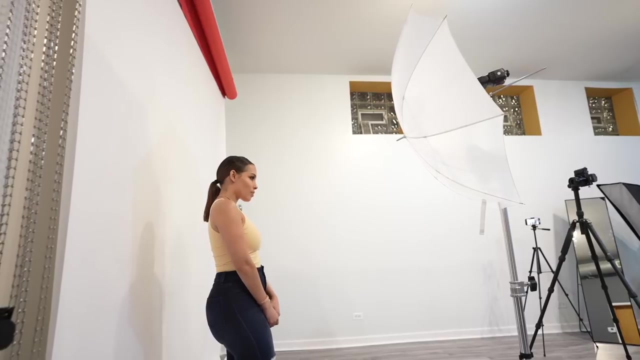 do this, you are going to be capturing the shadow right next to her in the photo. Depending on your personal taste, you may or may not like this look. I personally think it looks okay When you ask the model to take a couple steps away from the background. I would say around a foot away. you're going to be getting 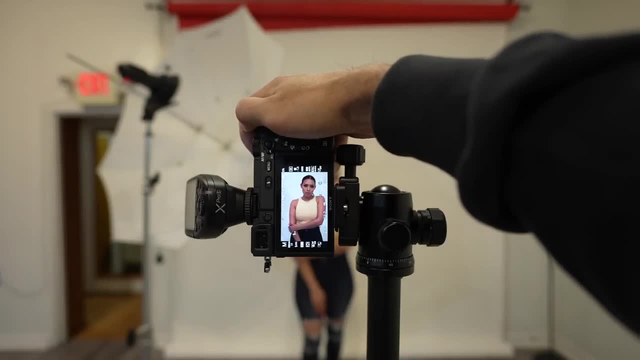 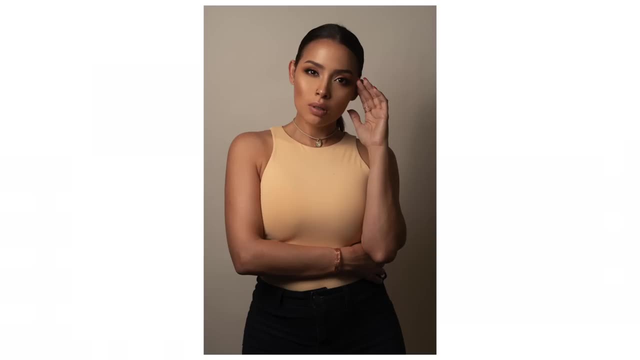 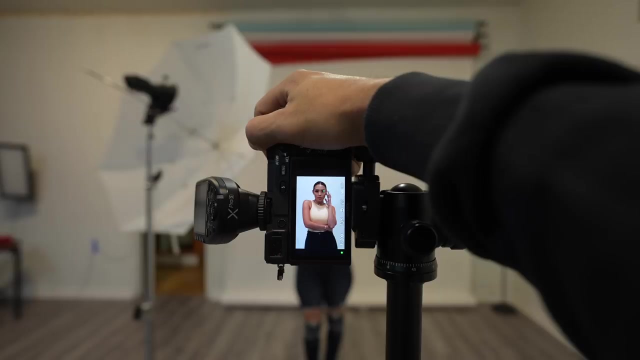 a softer, more pleasant shadow fall off onto the backdrop And, in my opinion, it looks better than when she was up against the wall. Now, when you ask the model to stand about four feet away from the backdrop or the wall that you're using, you're going to be eliminating her shadow from the photo. 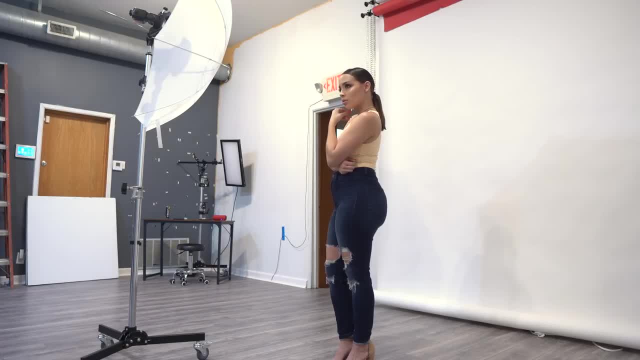 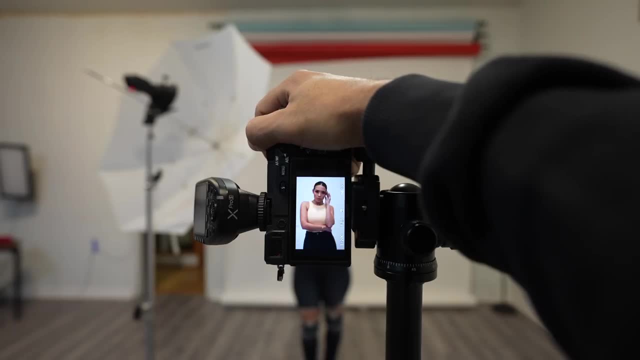 And, unlike a more directional light source, an umbrella is spreading the light in every direction And you're going to be getting a nice soft grading of light on the background. In my opinion, this one looks best, but none of these are bad. It just depends on the look that you want for your. 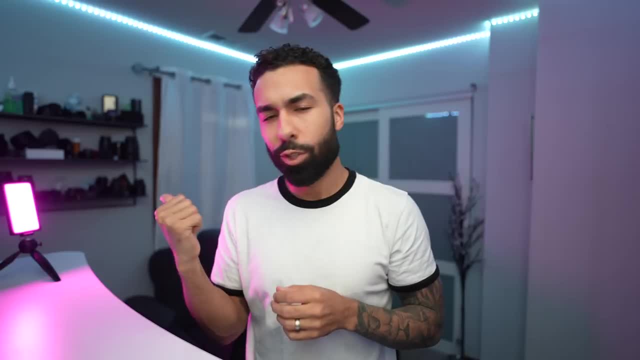 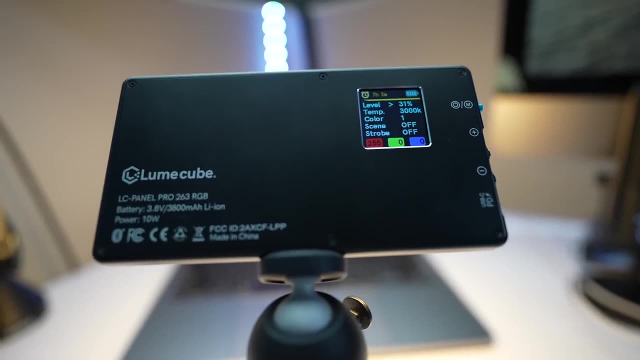 photo. Okay, Since we're on the topic of lighting, do you see that nice purple kicker light that I got going on here? Let me tell you about this new RGB light that Lume Cube just released. It's called the Panel Pro and it's the largest light panel in their lineup currently, And it 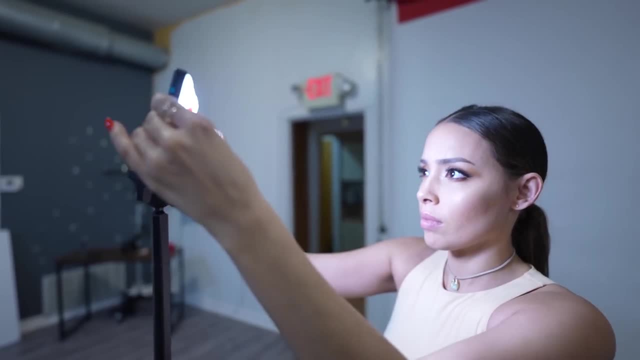 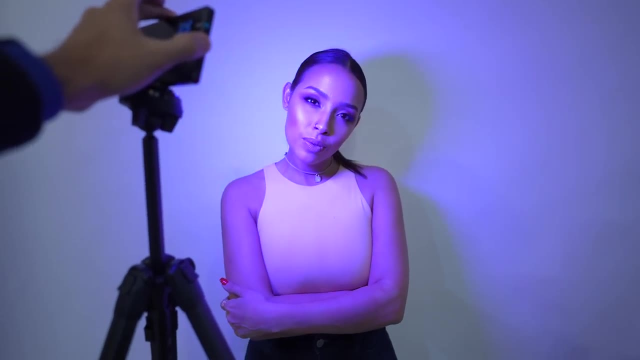 produces some really nice soft light. This is a very slim and portable light. It's a very slim and portable RGB light designed for photographers and videographers. This RGB light gives you 360 color options with a color temperature range from 3000K to 5700K. It has some creative modes. 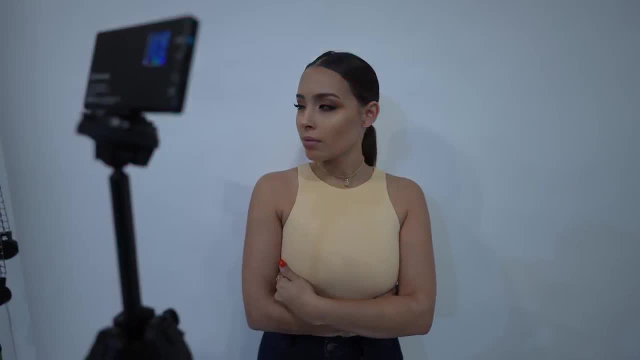 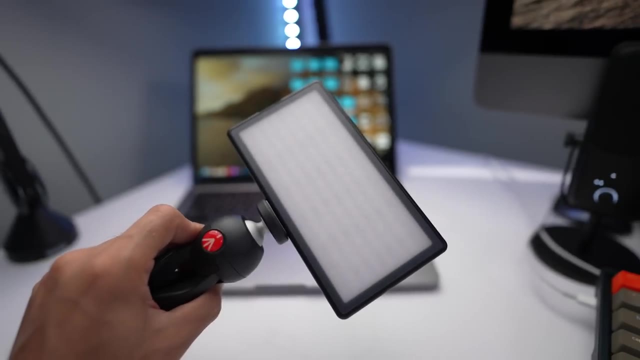 for video like it emulates what a siren would look like a fire and lightning. It weighs 200 grams, has four quarter thread mounting options and has a really long lasting battery. This light is Bluetooth compatible and using the Lume Cube app, you'll be able to control as many of these. 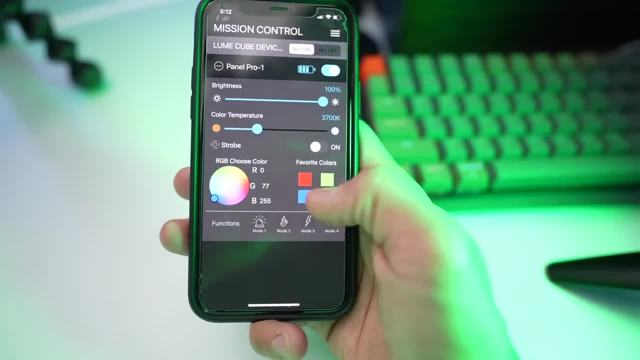 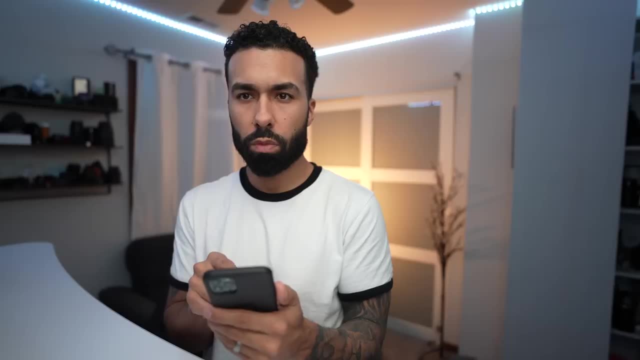 panels as you want, all while being able to tweak your color and settings from your phone. Just by testing it here in my office using the app, I think I found myself a new light for my studio, either as a kicker or a background light to set the mood in. here, This Panel Pro will be 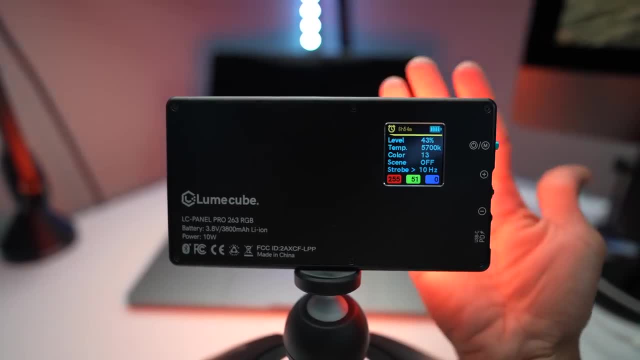 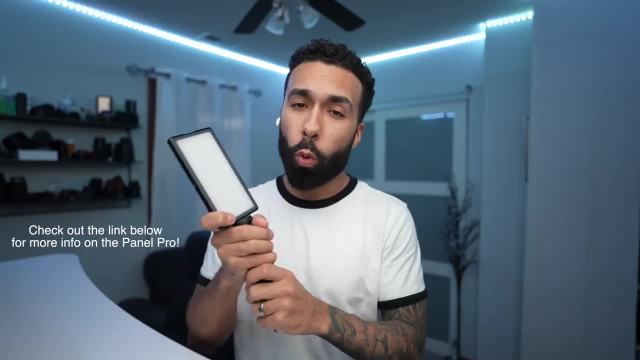 available at a discounted rate of $199 in their limited stock launch. Once those sell out, it's going to be available in early December for $229.. So you don't want to miss out on saving some money. click the link down below to see more on Lume Cube. 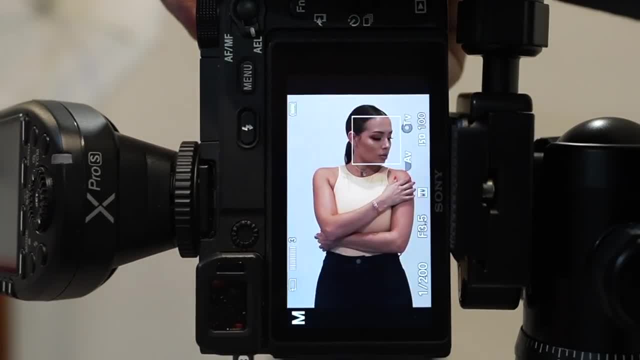 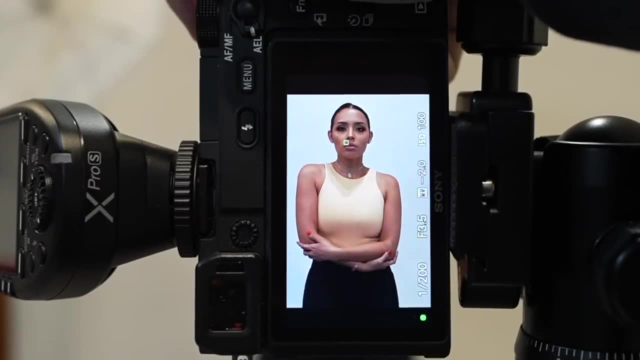 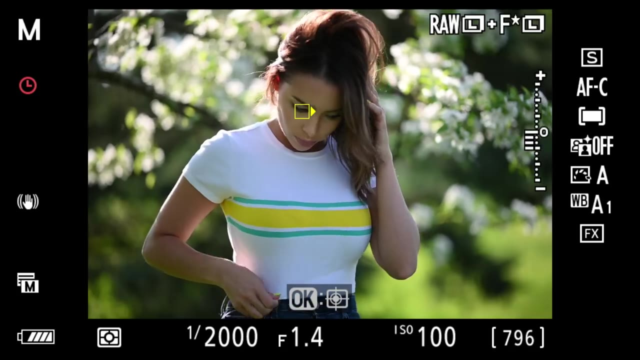 So let's go over the settings that I used in this video. The settings that I used were ISO 100, f3.5, and 1200 shutter speed, And my intention was just to kill the lights that I have in my studio, so it didn't affect my exposure. I used ISO 100 for the 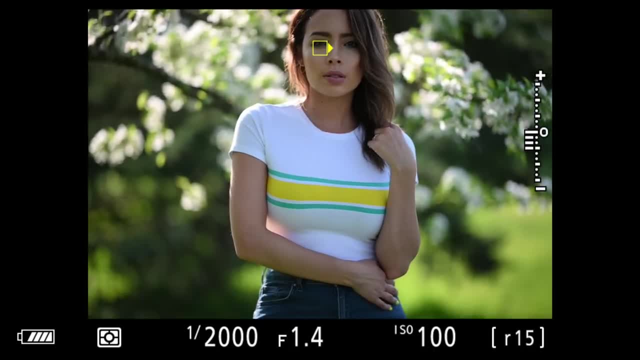 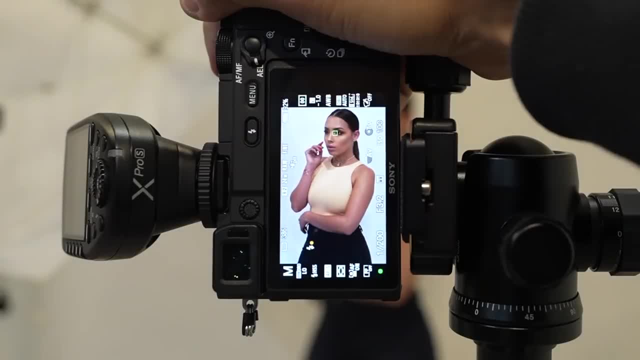 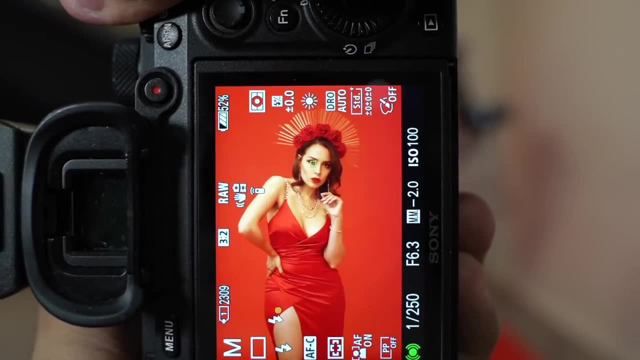 aperture: I used f3.5 aperture. I used f3.5 aperture. This is an f1.8 lens, but for studio work you don't need to shoot wide open. I prefer to shoot at a smaller aperture so I can get more in focus and get more sharpness. 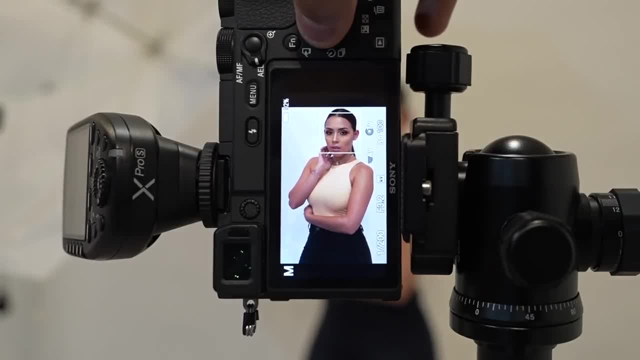 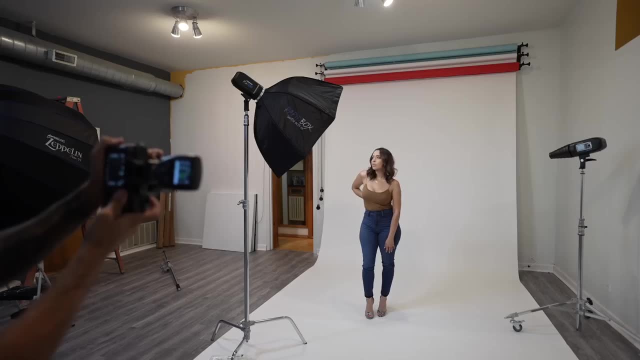 The beautiful thing about this flash is that it can shoot high speed sync and I can use any shutter speed that I want. If I can, I would stay under the camera's flash sync speed because high speed sync puts extra strain on your flash and I didn't realize that on this camera it was 1: 1: 60th.